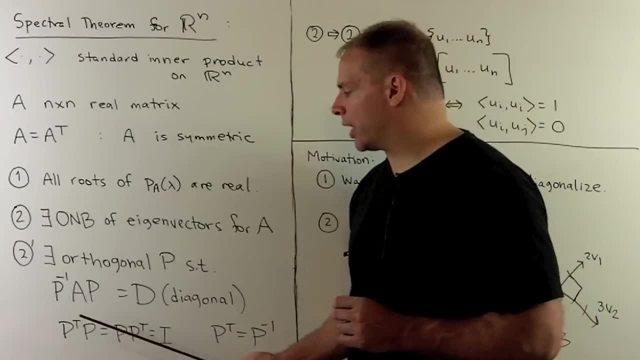 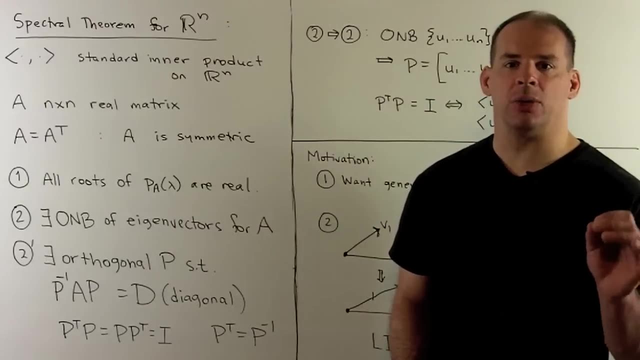 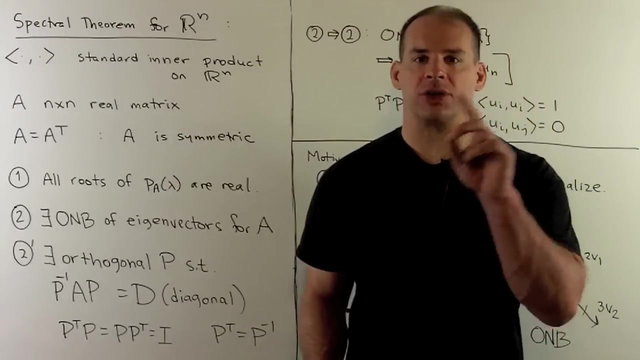 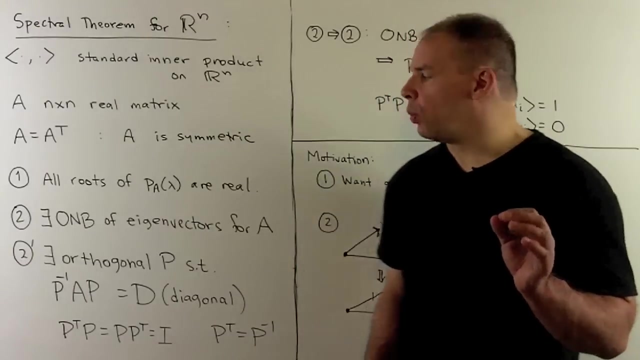 Recall orthogonal means: P transpose times, P equals P, P transpose equals the identity matrix, or P transpose equals P inverse. So the idea here: if we apply P to our vector space, then the interproduct will be preserved. Now, why are these two statements equivalent? First note: if I could put A into diagonal form. 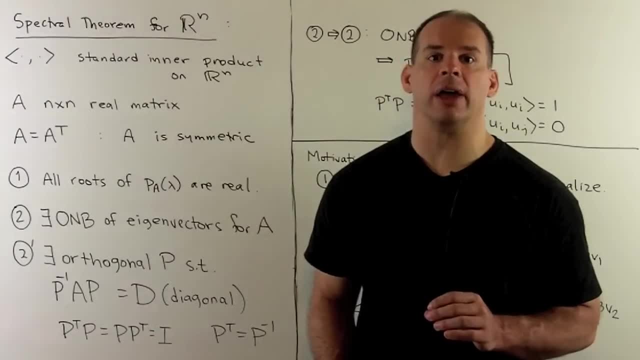 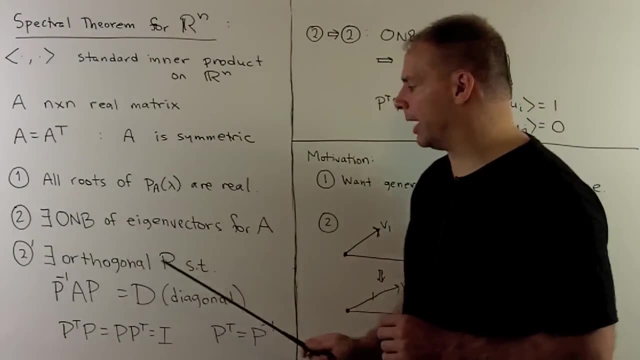 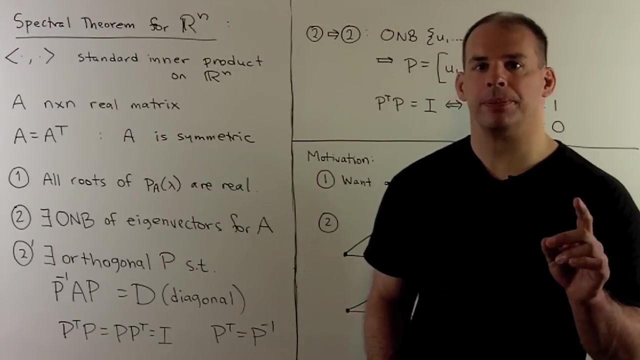 that's equivalent to the statement that we have a basis of eigenvectors for A. So we just need to explain the connection between the orthonormal basis and the orthogonal matrix P. Now A can be put into diagonal form using P. What we'll do is we'll have A On the right. 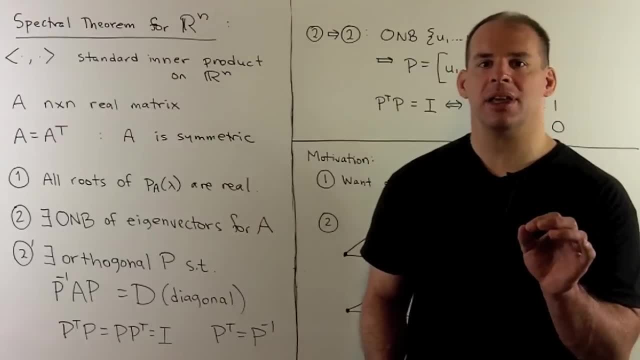 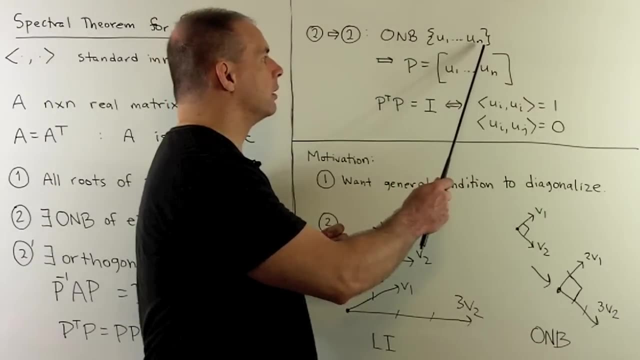 we're going to put the matrix P, which has as its columns the eigenvectors for A, So let's call those U1 through Un. So P is going to be U1 through Un. We have U1 through Un as our. 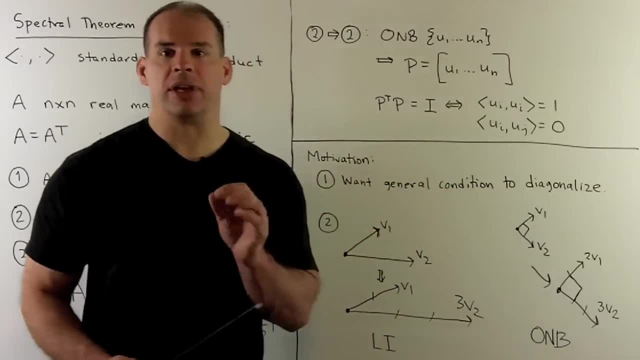 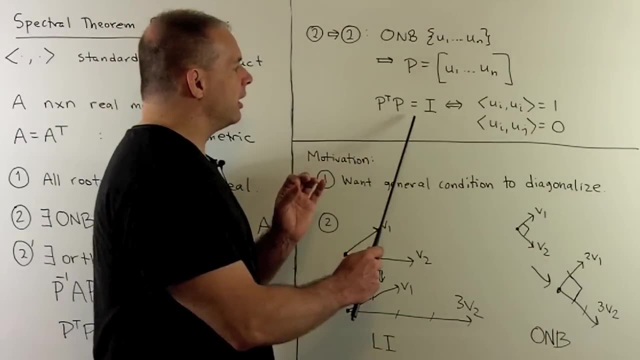 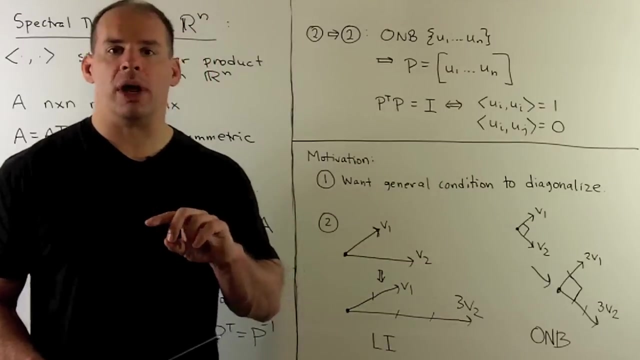 orthonormal basis. Now the condition P transpose, P equals the identity. We're just interpreting the row times column products here. So what's happening with these row times column products? Well, when I transpose, okay, that row times column product just becomes interproduct of two of our columns. 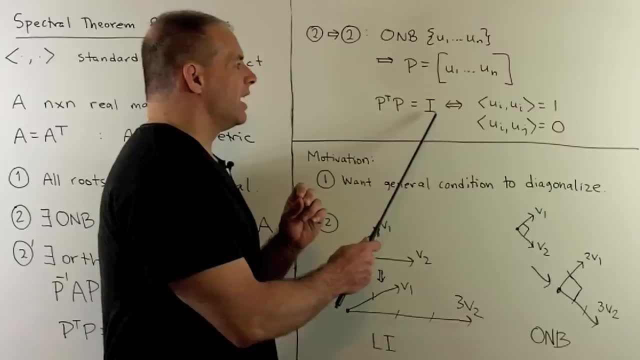 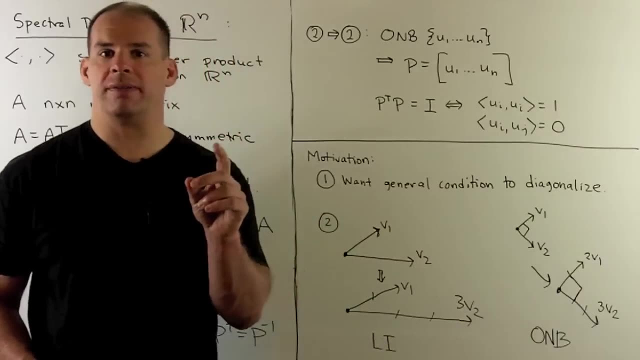 So to have the P transpose, P equals the identity, is equivalent to saying, okay, the interproduct of column with itself is equal to 1.. So we have unit vectors And if we take distinct columns, we're going to have the. 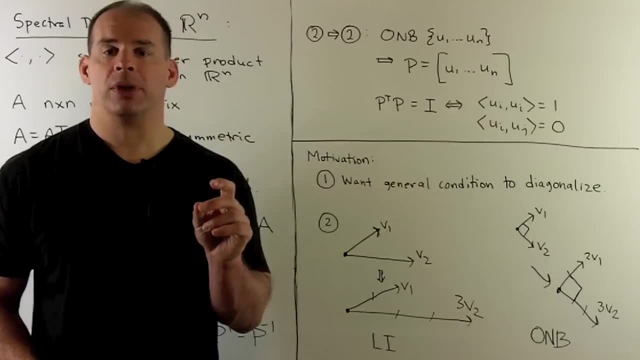 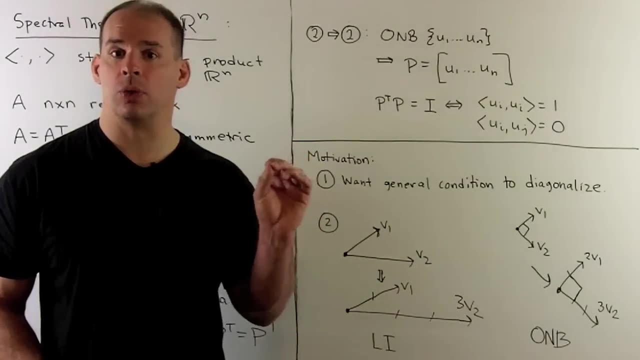 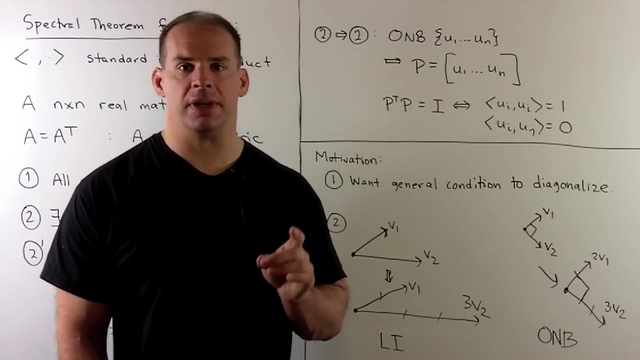 interproduct is equal to zero, So orthogonal. So our basis of the U's is an orthogonal basis of unit vectors or an orthonormal basis. Now, the spectral theorem has big applications in math and physics, For here we'll note some. 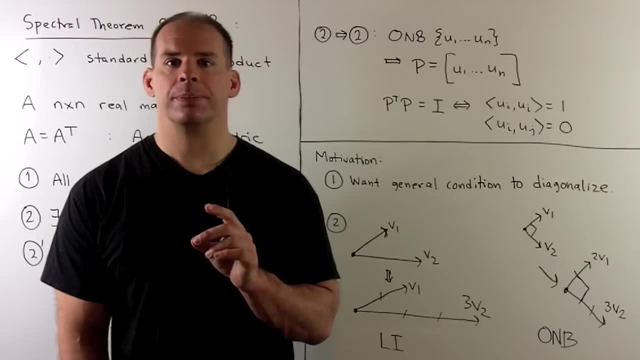 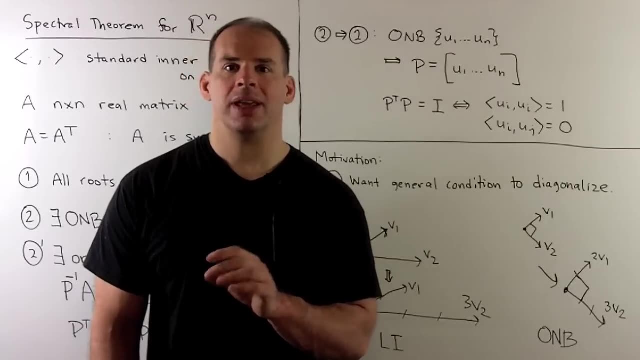 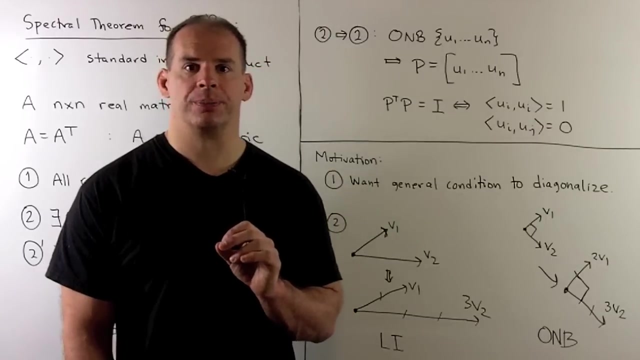 immediate advantages. First, we have a condition for diagonalizability, So A is real symmetric. Then we can automatically put A in diagonal form. We can't do that for a general real matrix. Two things that get in the way: The eigenvalues of our matrix. 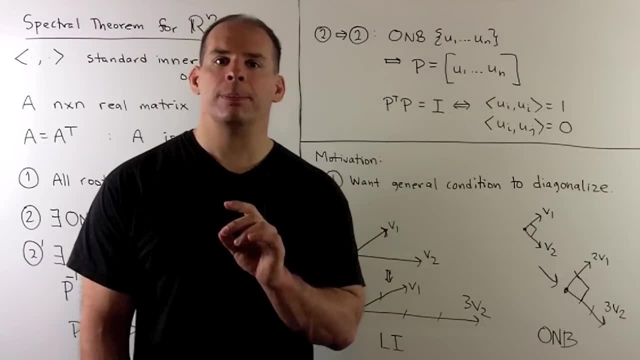 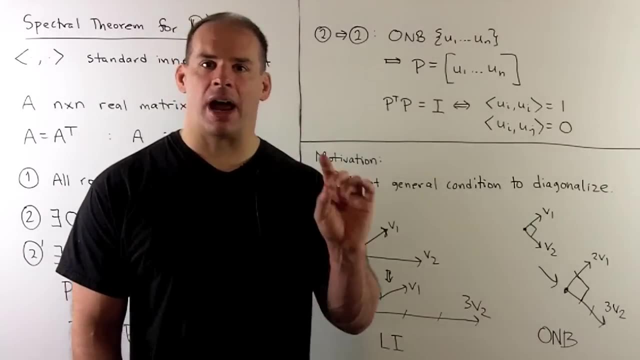 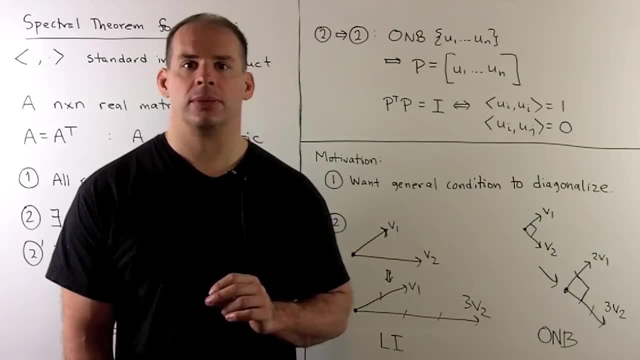 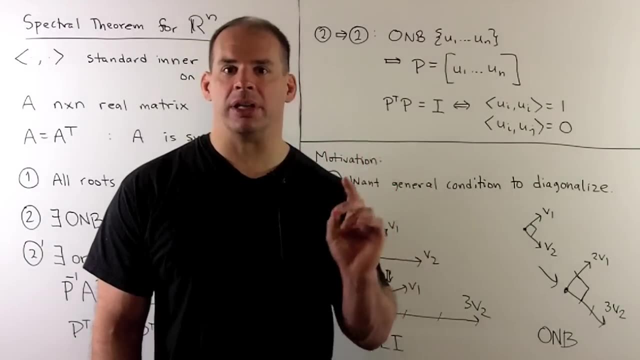 So when A is real symmetric, the spectral theorem guarantees that A is real. So when A is real symmetric, the spectral theorem guarantees both conditions. Next, we could think of the spectral theorem as the next step in diagonalizability. So if we know how to diagonalize a matrix, we can add an. 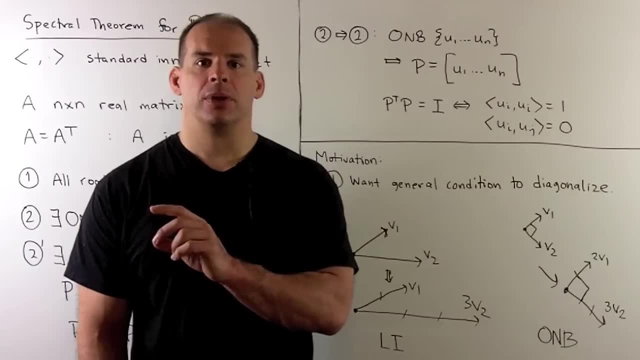 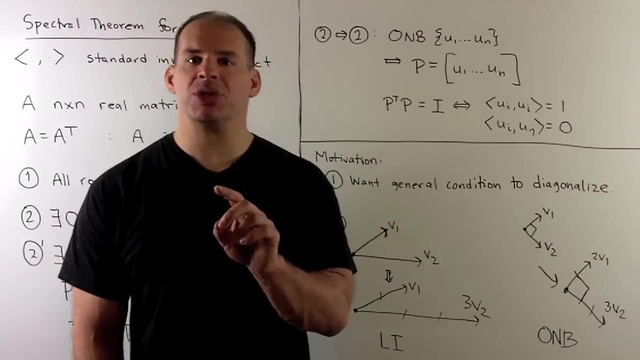 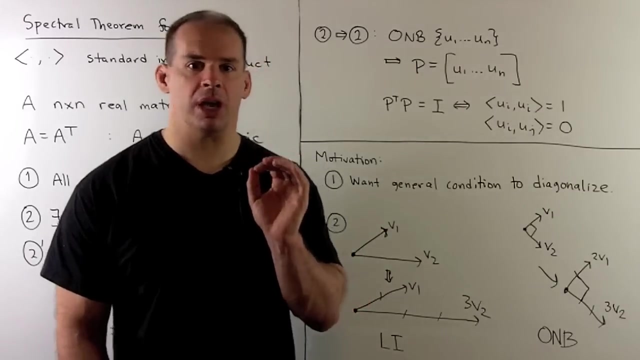 interproduct to the picture. then we would ask: when can we diagonalize without disturbing the inner product? So that would mean we want to change a basis that's represented by an orthogonal matrix. So that happens with the spectral theorem. Now to look at pictures. when we have general 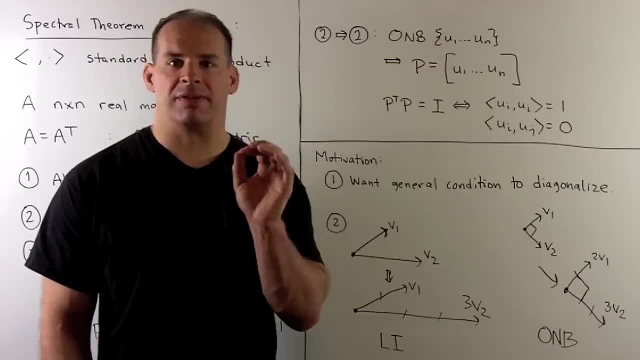 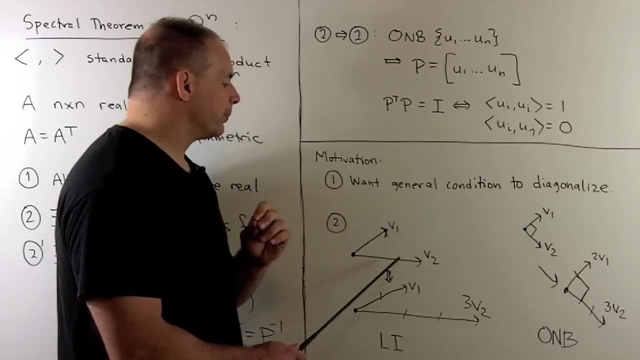 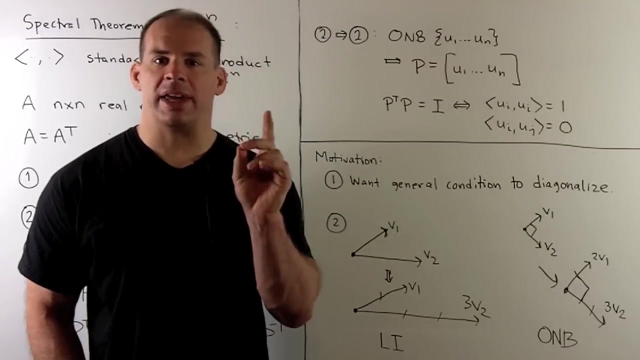 diagonalization, all we're guaranteed is a basis of eigenvectors, which just means linearly independent. So while I could make these vectors unit vectors, that's not going to guarantee that they're perpendicular. If we have the spectral theorem, then we're guaranteed an orthonormal basis. So again we can make. 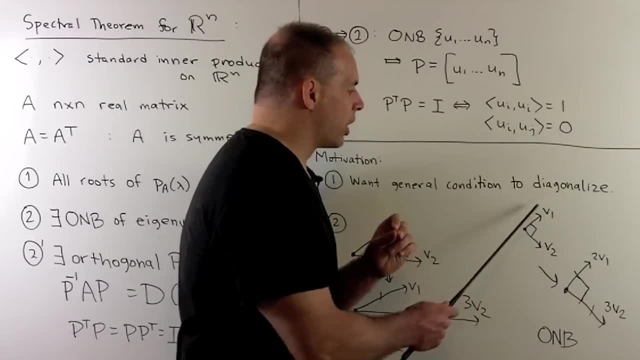 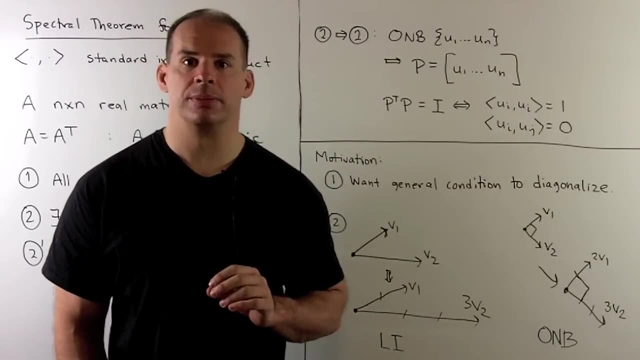 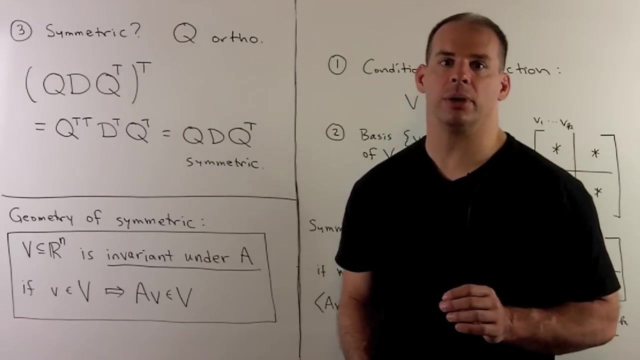 them unit vectors. but we're guaranteed to have this right angle in there. So that makes for a nicer picture and it also makes for cleaner computations. Third, what's the evidence that a symmetric matrix has such nice behavior? So we'll work backwards. Start with Q- orthogonal, We'll have a diagonal matrix, D. 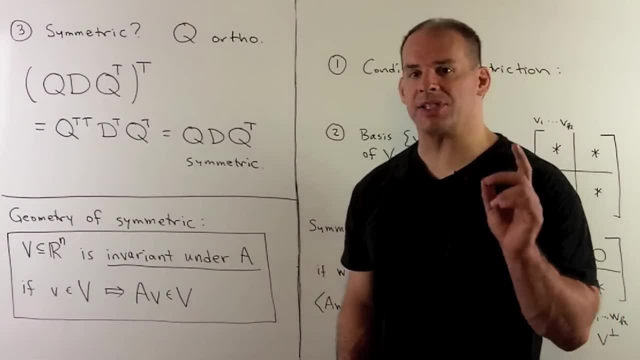 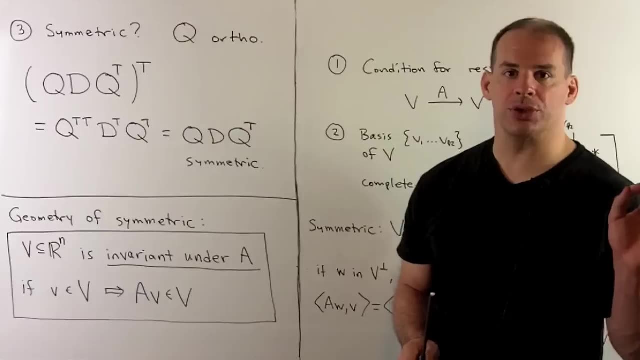 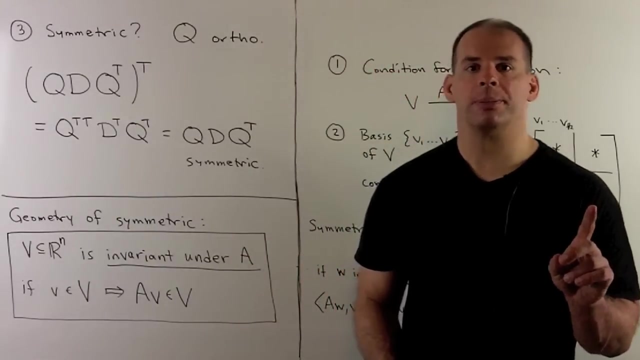 I'll conjugate D by Q to show that that's symmetric. So we'll have Q D, Q inverse- Q is orthogonal, Q inverse equals Q. transpose: If I take the transpose of this product, the rule is we will reverse the order. Take the. 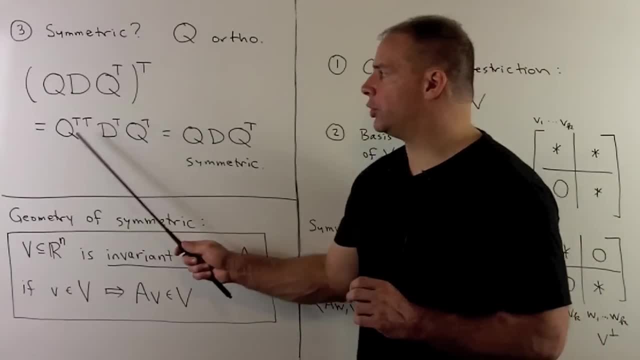 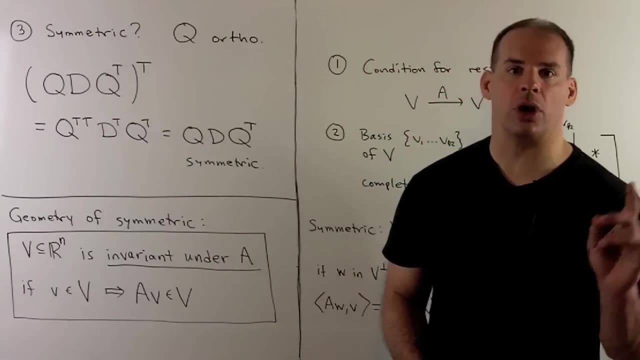 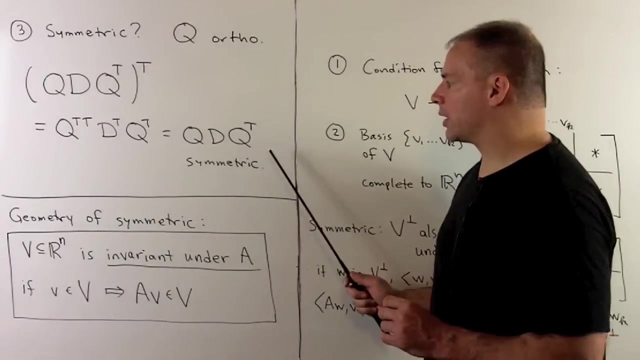 transpose of each term. So I'll have Q transpose, transpose, D transpose, Q transpose. If I take the transpose twice, we get our original matrix. Since D is diagonal, D transpose is equal to D, So we get our product back. 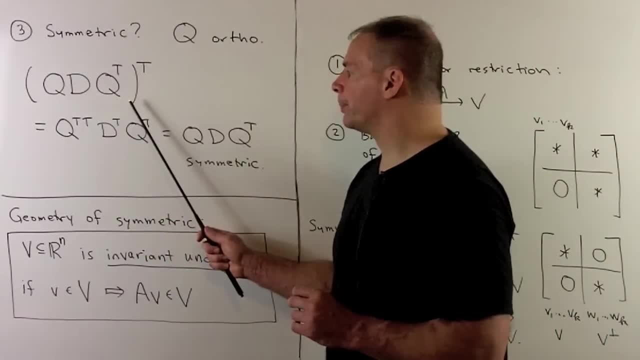 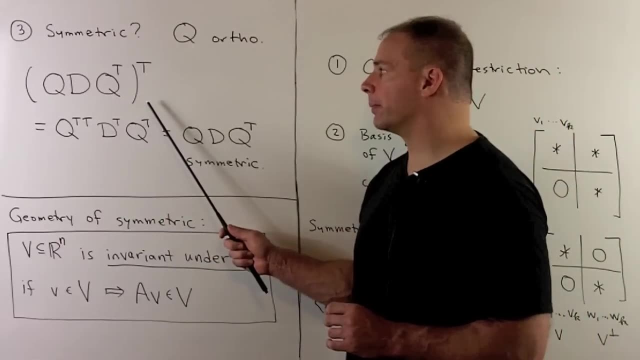 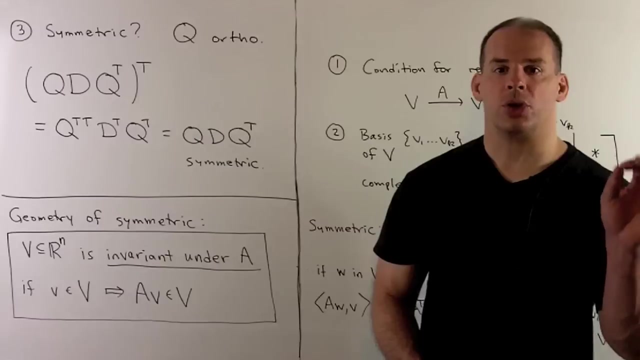 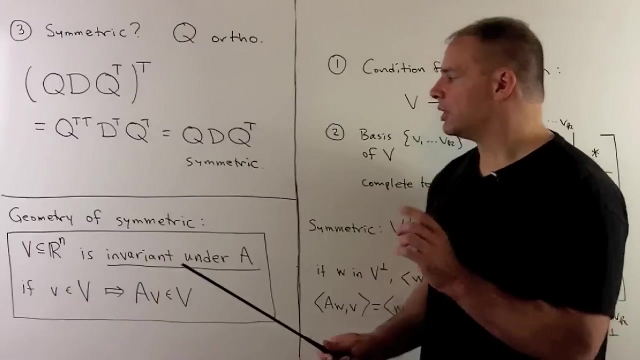 So that means this matrix is symmetric and we have some evidence that every symmetric matrix might be able to be written in this form. Now let's start the proof. So our first step is to understand the geometry of a symmetric matrix. So we'll start with definition. If we have V, a subspace, 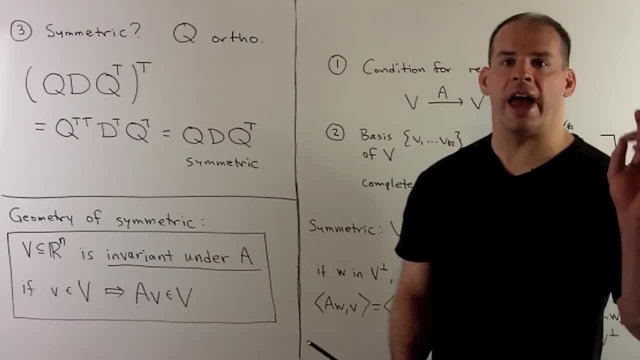 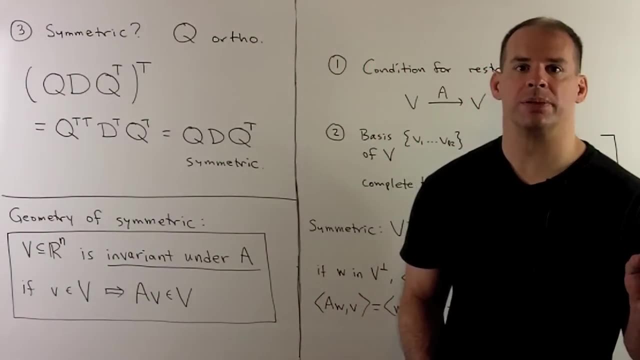 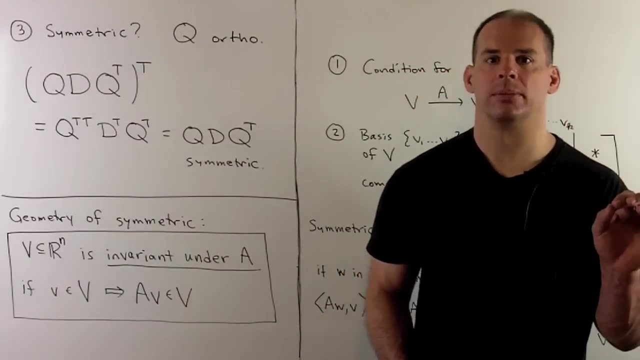 of Rn, we'll call it invariant under A, if whenever V is in our subspace, A times V is also in our subspace. So the idea here, if we apply A to our subspace, just carries it back into itself. How should we think of our definition? First, we're looking for 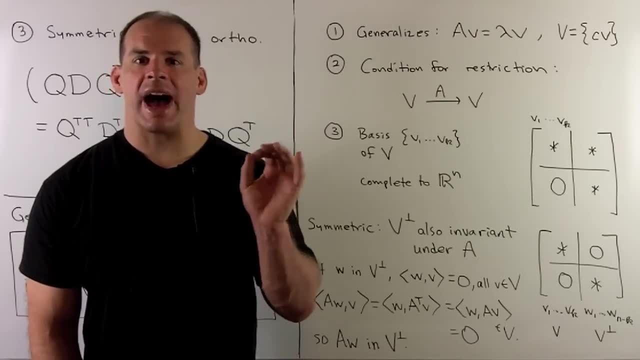 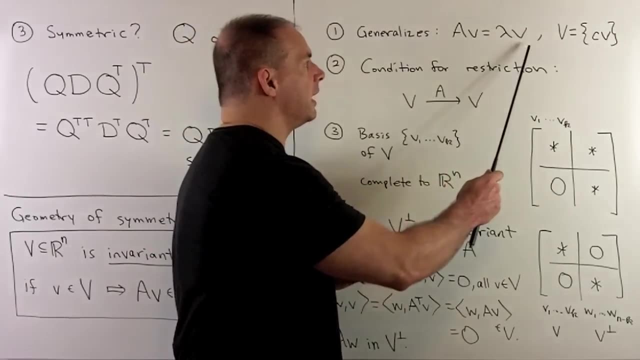 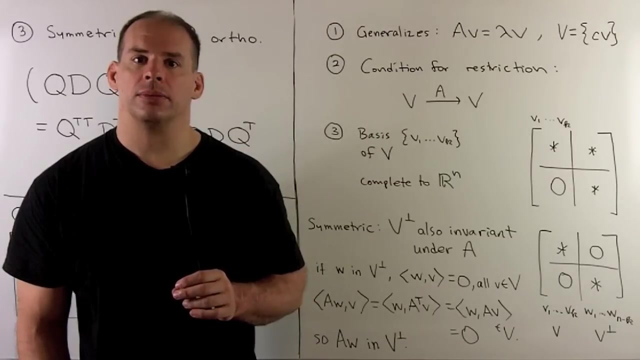 an example of a subspace that's invariant under A. Think eigenvectors. So if A has a nonzero eigenvector, V, Av is equal to a multiple of V. the subspace formed by all multiples of V will be invariant under A. Second invariance under A is the precise. 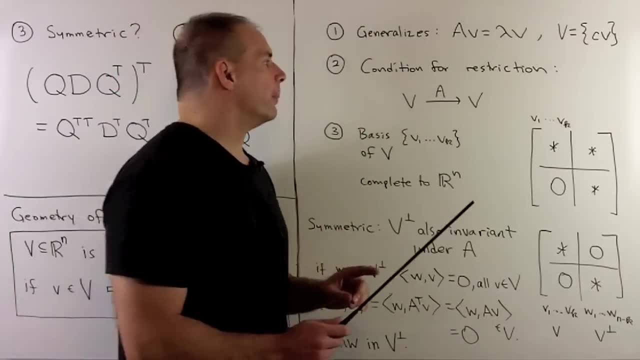 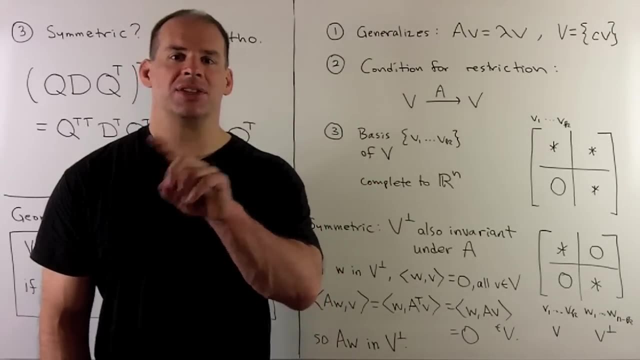 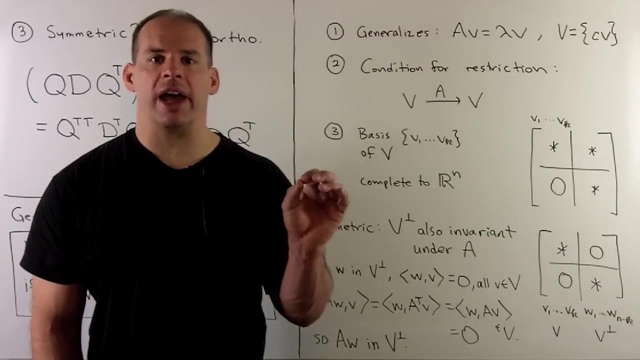 condition that we want for restrictions. So if we think of A as a map from Rn to Rn, I can restrict that map to any subspace in Rn. To be a proper restriction, we'd want that subspace to get carried back to itself under A. That's precisely the condition. 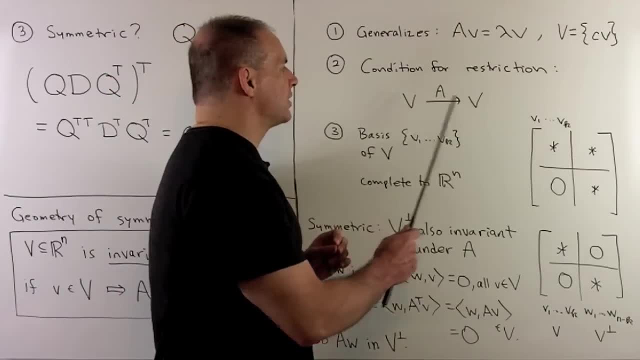 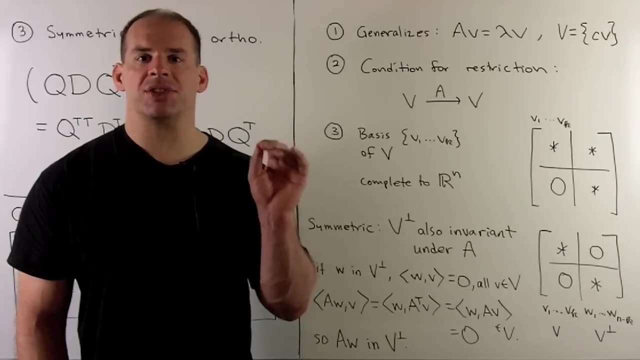 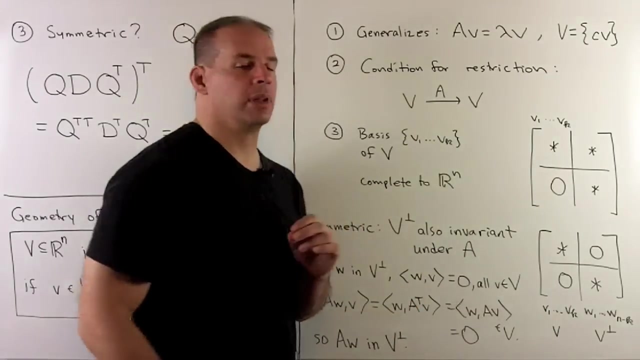 of invariance under A. So we have that V gets carried to V under A. Third, let's choose a basis for our invariant subspace, say V1 through Vk. I can complete that to a basis for Rn and then I can consider the matrix for A with respect to this new basis. 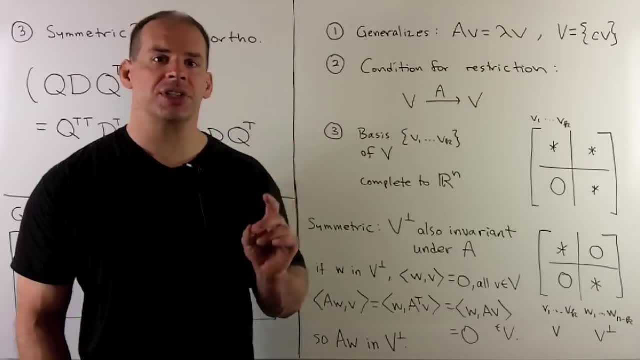 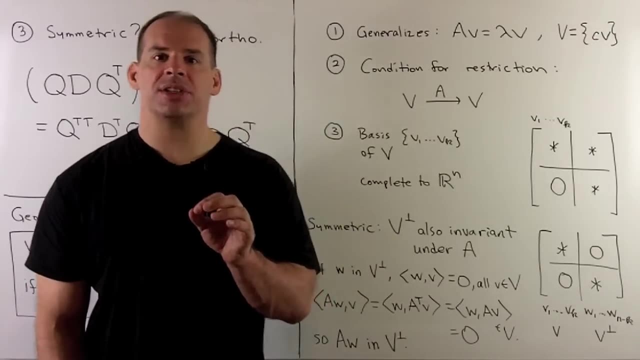 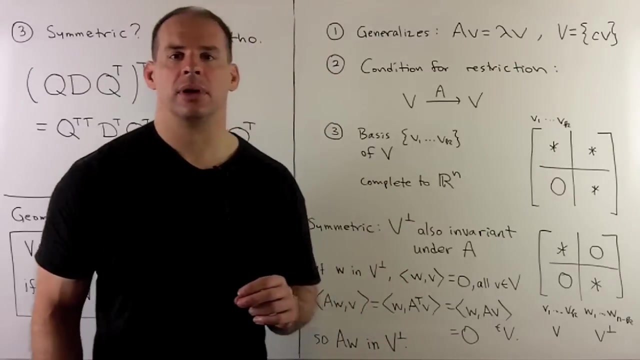 Now the recipe for forming the new matrix. We're going to apply A to each basis vector. That gives us a linear combination in our basis We peel off the coefficients and that gives us the column that goes with our basis vector. Now, if we choose a basis vector from 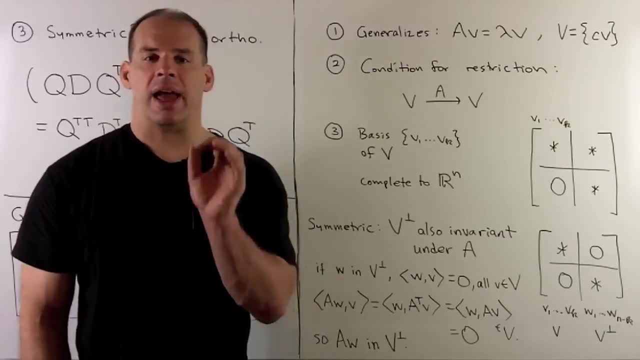 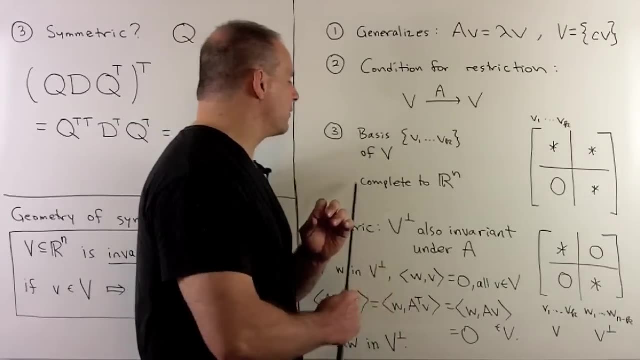 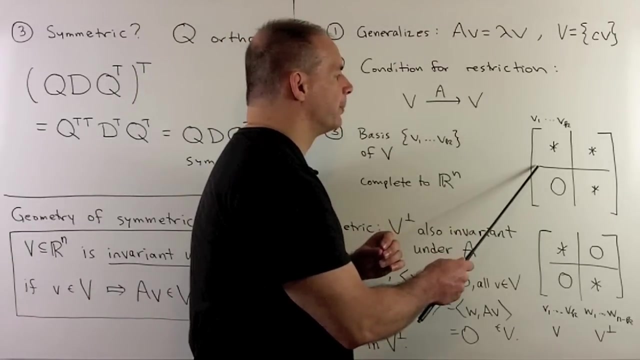 our invariant subspace, say V1, A is going to carry V1 to a linear combination in the Vs. That means the coefficients on the rest of the basis vectors will be zero. So the column for V1 will have k entries and then we'll have all zeros And that'll hold for V1 through. 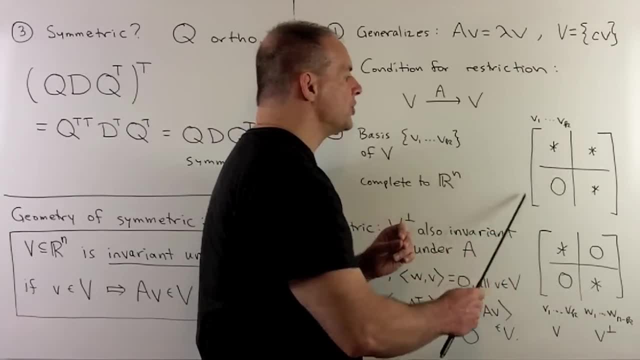 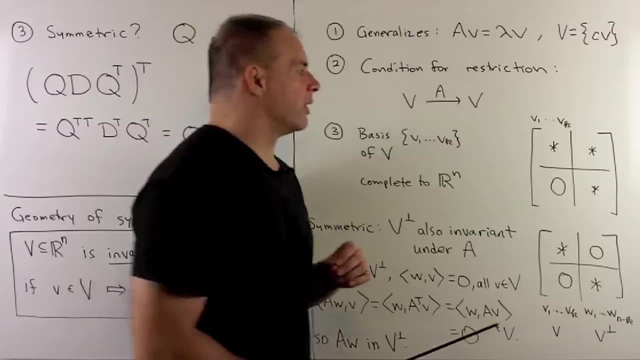 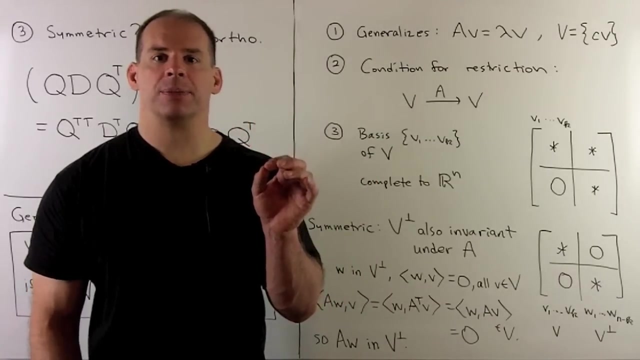 Vk. So I get a k by k block and then all zeros below. For the rest of the basis vectors we have no information. so all we know is that we have a block here and a block here That says if we have an invariant subspace, we choose our basis correctly. the new matrix for A. 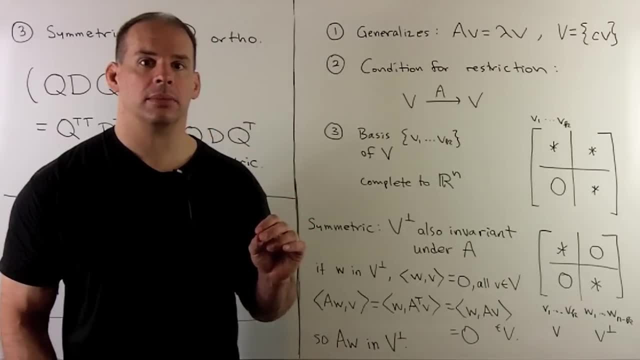 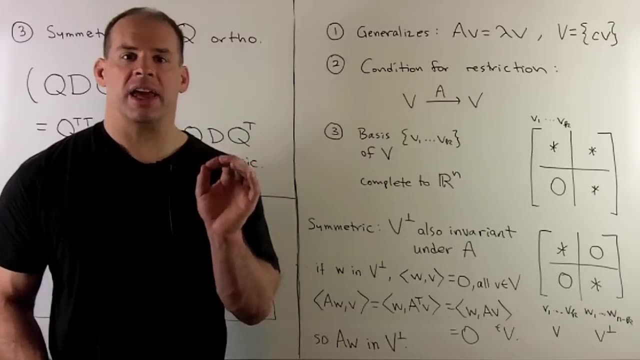 will be block upper triangular. Now if A is also symmetric, we could say a little bit more. So in this case the orthogonal complement to V will also be invariant under A. So let's choose a basis for that, say V1 through V sub n minus k. So if I put that together, 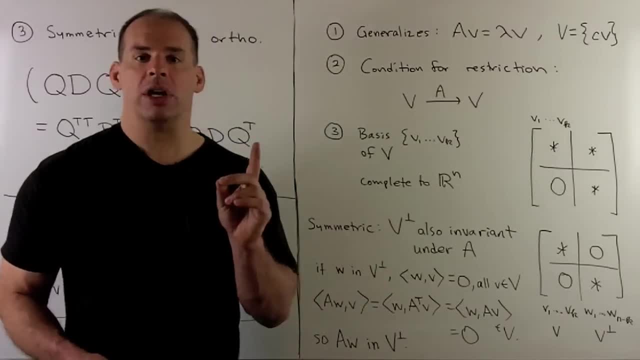 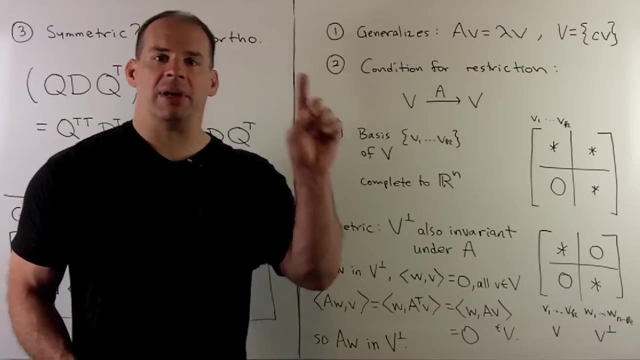 with the A we get a basis for Rn And we note by invariance, if I apply A to say W1, we get a linear combination of the Ws. So that means the coefficients on the Vs are going to be. 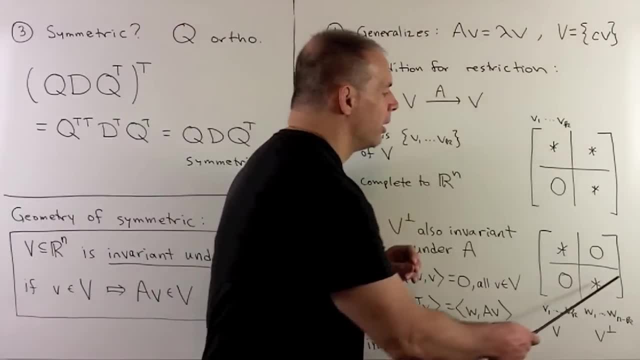 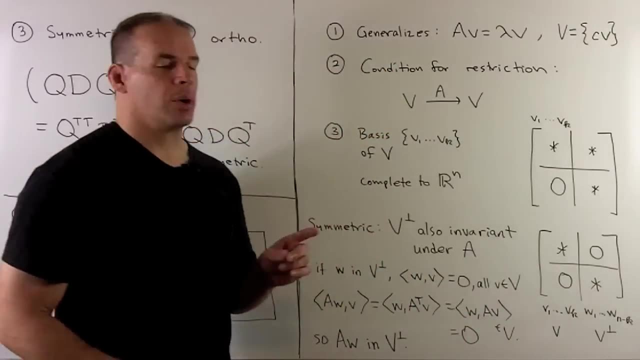 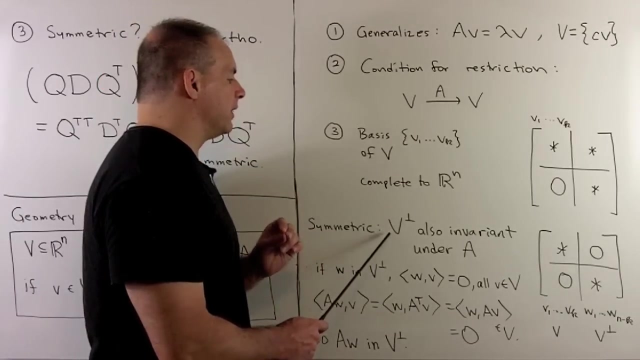 zero. So we're going to have another block which is possibly non-zero, with all zeros above. So in this case we're going to get a block diagonal matrix. Now we have to show that the orthogonal complement to V is also invariant under A. So what are we trying to show here? 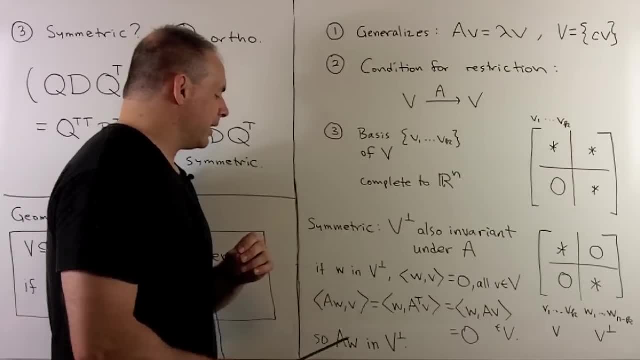 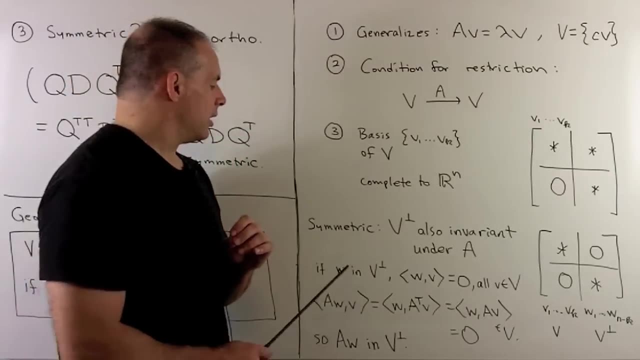 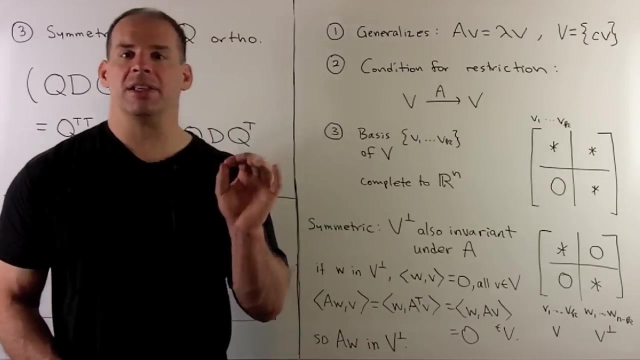 We're showing. if W is in the orthogonal complement, then AW is also in the orthogonal complement. Definition of the orthogonal complement: W is in the orthogonal complement if the inner product of W with V is equal to zero for all V in the subspace V. So we're going to check. 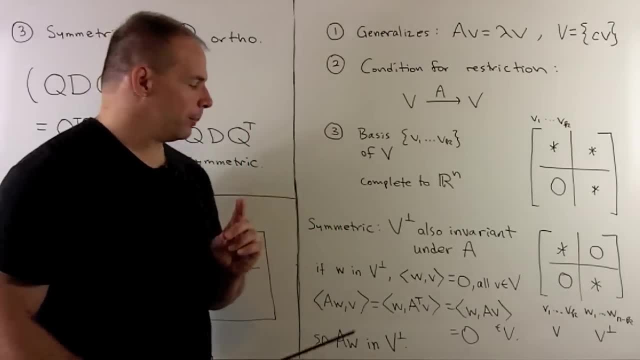 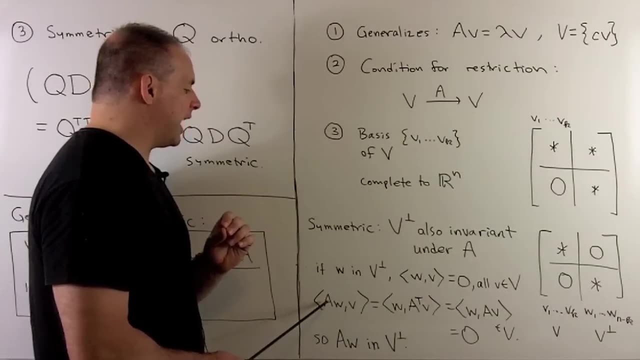 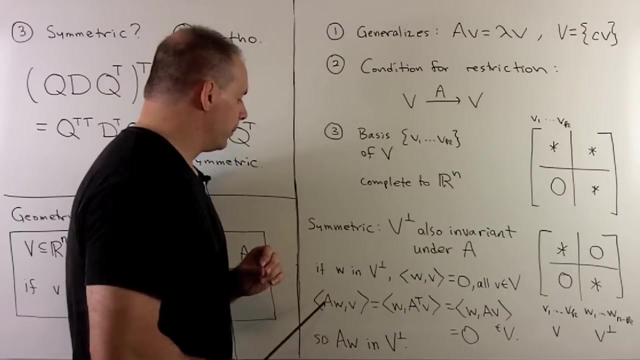 that with AW and sub space V. So we're going to check that with AW and sub space V. So if I take AW inner product with V, for any V in the subspace V, we're going to push the A to the other side by the rule for how we transpose in the inner product. So that goes. 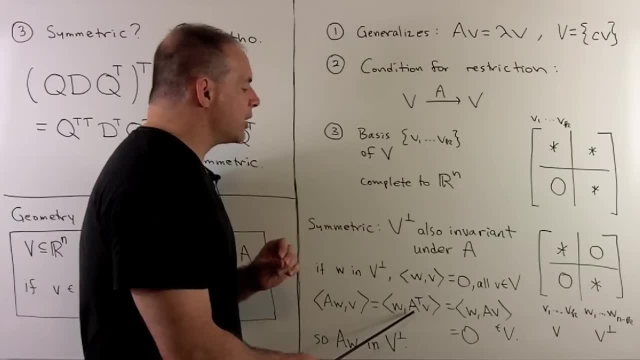 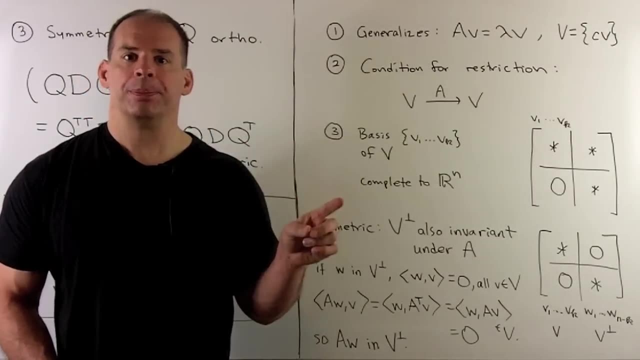 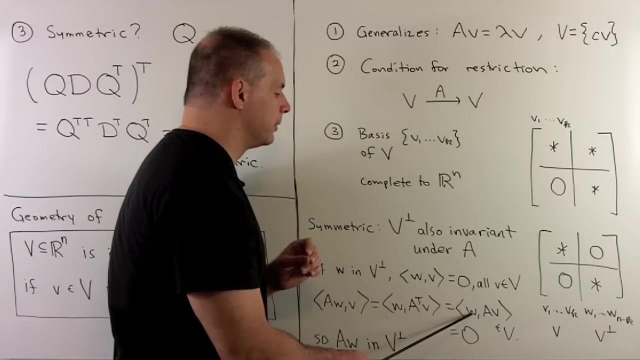 over as A transpose. Now, because we're symmetric, A transpose is equal to A AV. by invariance of V is in the subspace V, So the inner product of W with AV is going to be equal to zero because W is in the orthogonal complement. So that says that AW is also in the orthogonal. 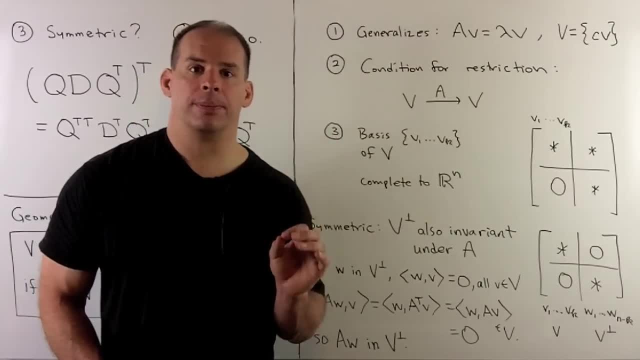 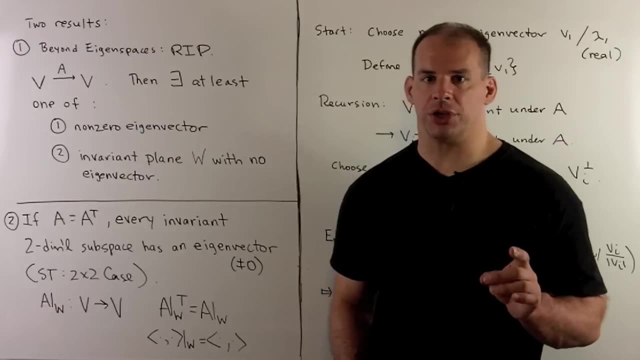 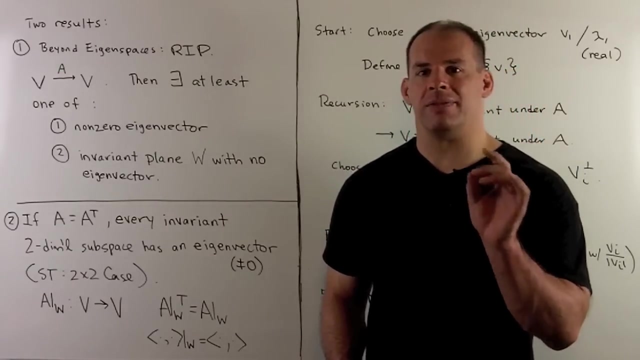 complement. So we have invariance under A To choose an orthonormal basis of eigenvectors for A. we use a recursive procedure. For this procedure to work we need the result that every non-zero subspace invariant under A contains a non-zero eigenvector for A. So 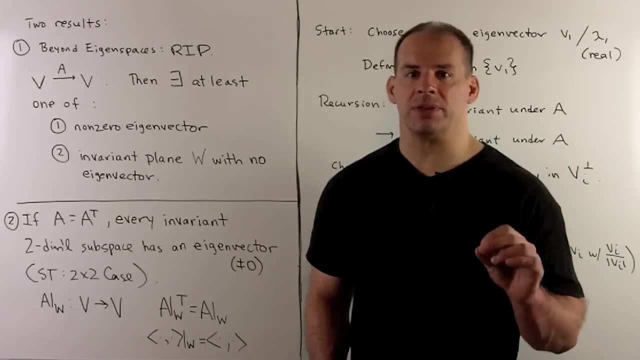 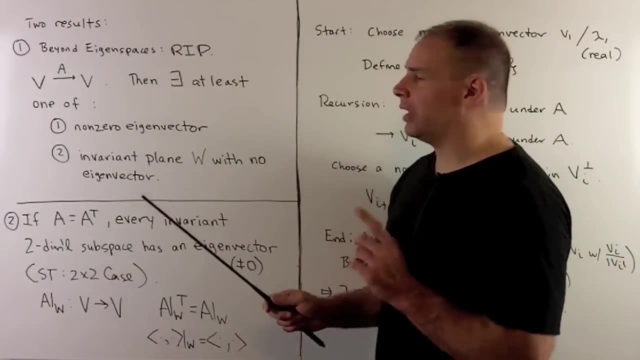 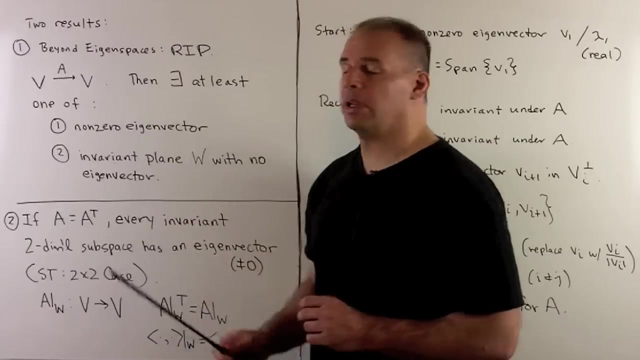 to see this I need to invoke two previous videos. First, for beyond eigenspaces, real invariant planes. if we have a non-zero subspace invariant under A call it V, so A carries V to itself, then there exists at least one of a non-zero eigenvector or an invariant. 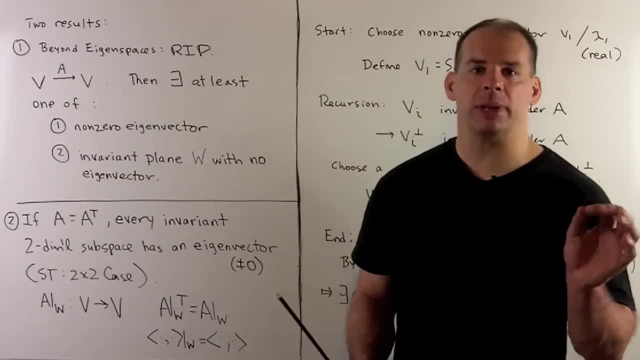 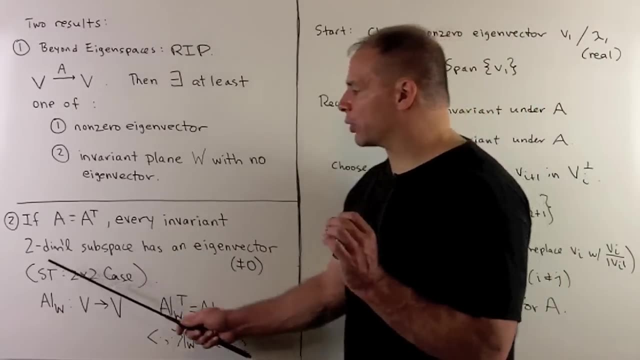 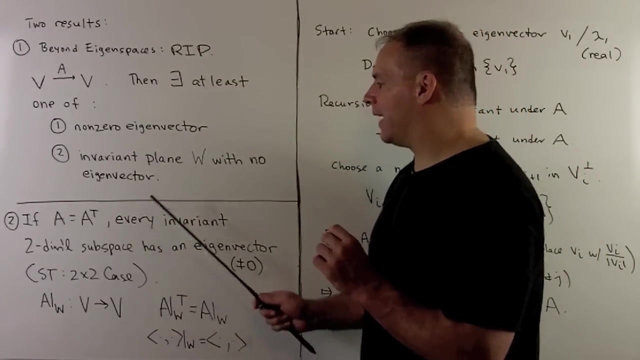 plane with no eigenvectors. Okay, by plane we mean a two-dimensional subspace. Now we can rule out the second case if we invoke spectral theorem for real matrices, 2 by 2 case. There we show: if we have an invariant two-dimensional subspace and we 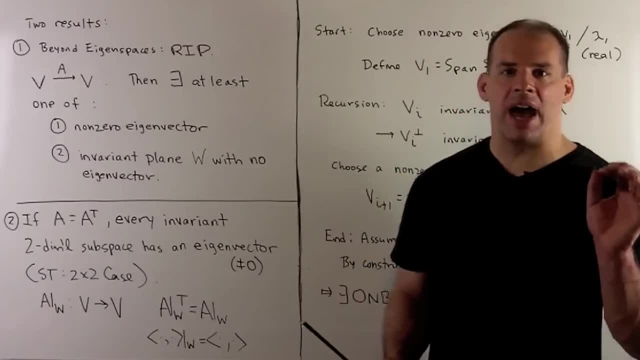 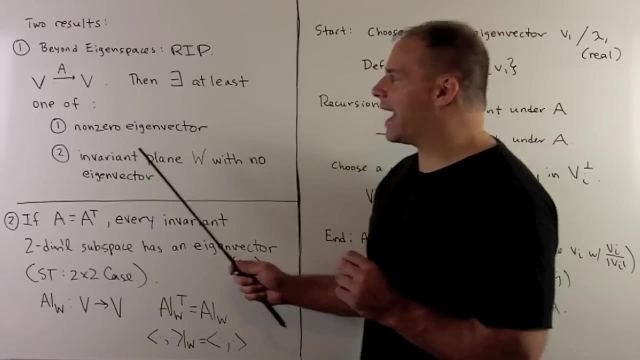 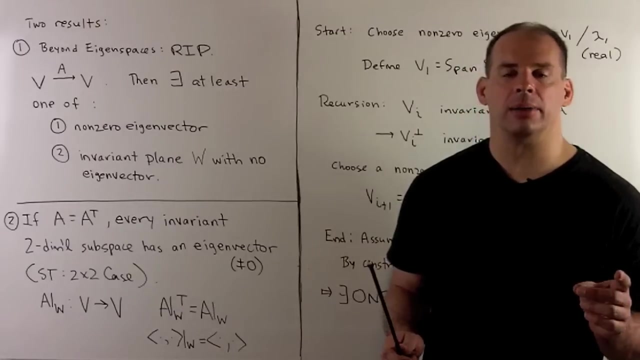 have a symmetric matrix, then we have to have an eigenvector. So that's going to rule out our second case here. So that means if I have a non-zero subspace invariant under A, we can always choose a non-zero eigenvector for a. Now let's define our 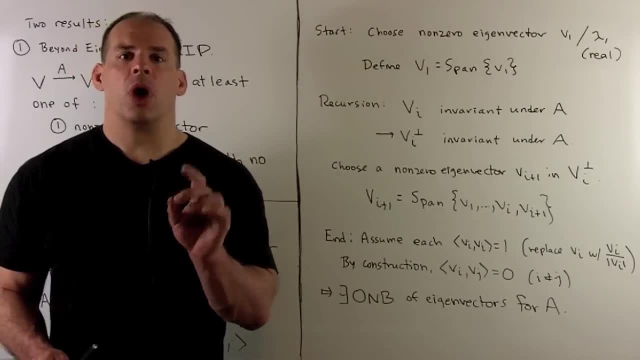 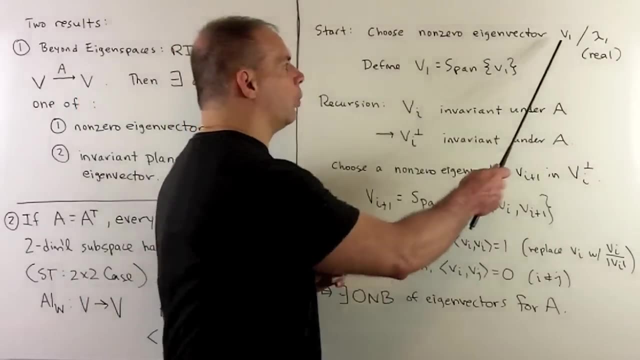 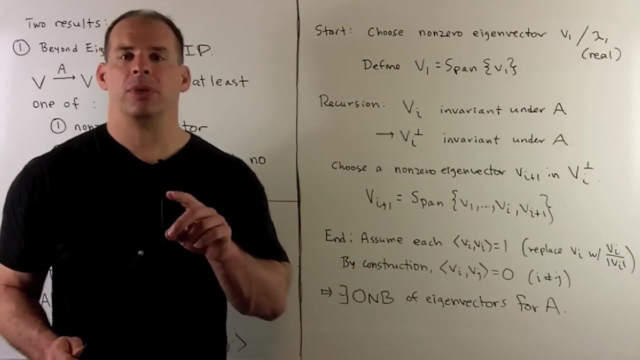 recursion. We start with: Rn is a subspace invariant under a, so we could choose a non-zero eigenvector. call it V1.. We'll call the subspace V sub 1 the span of V1.. Now for the recursive step. I'll assume that I have subspace V sub i in. 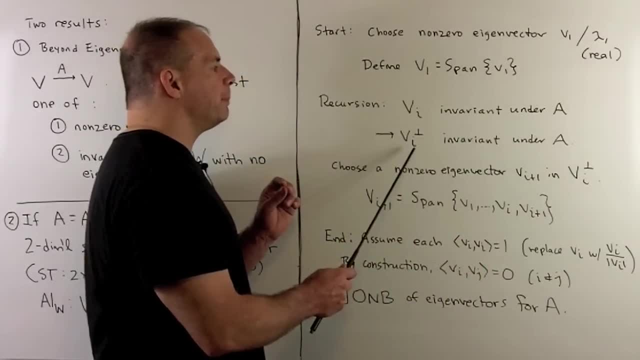 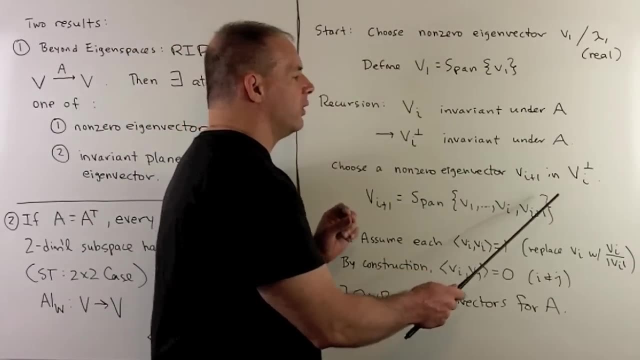 invariant under a. We could form the orthogonal complement, which will be also invariant under a. so we could choose a non-zero eigenvector, V sub i plus 1 in the orthogonal complement. Then I'll define V sub i plus 1 as the. 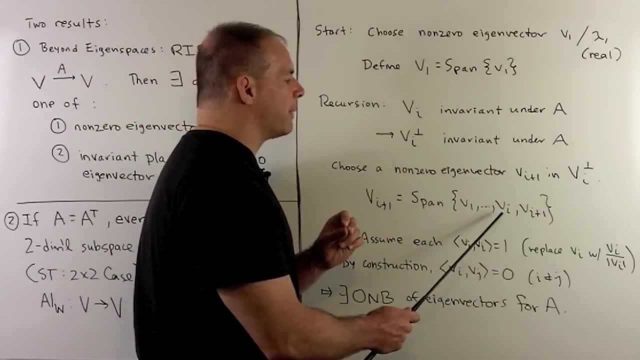 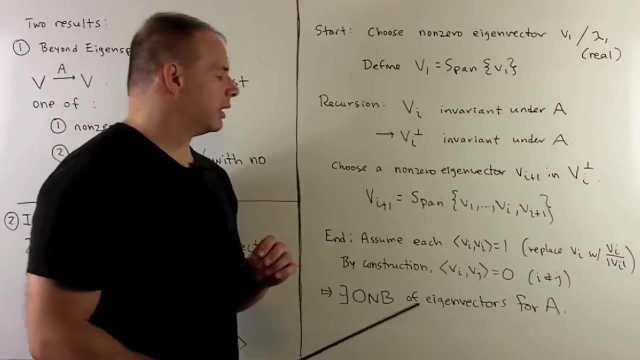 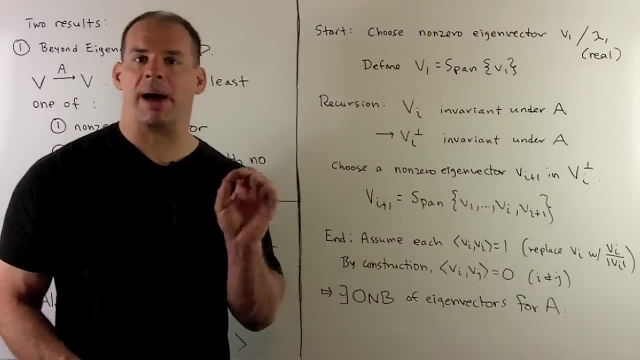 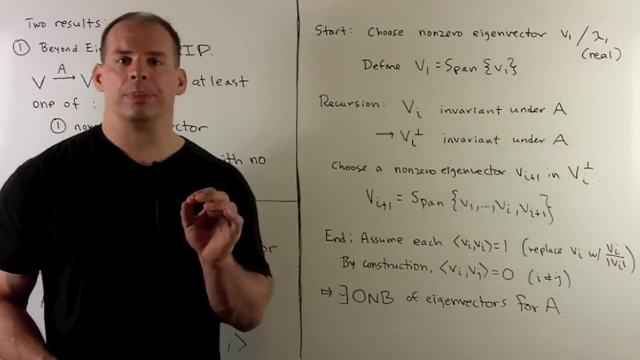 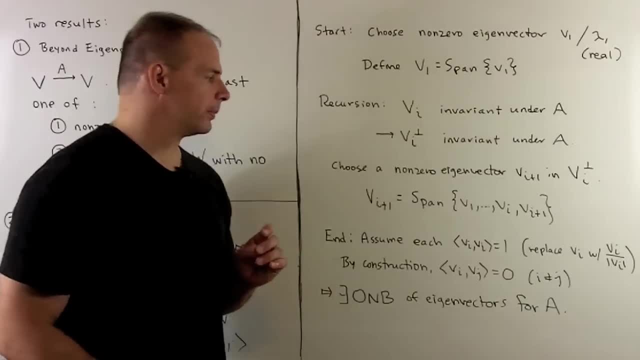 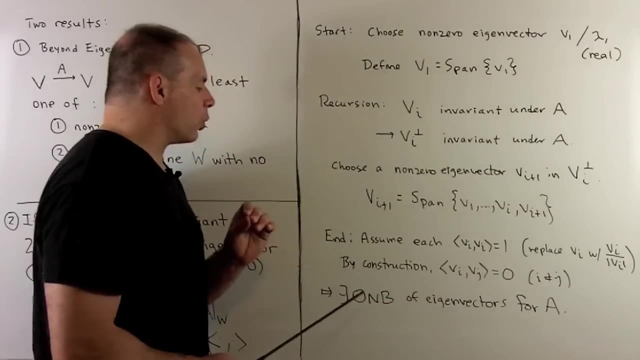 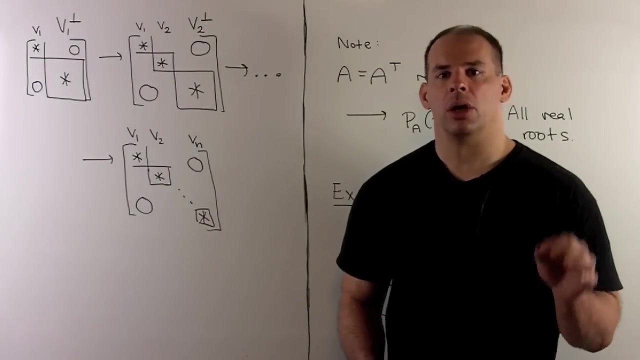 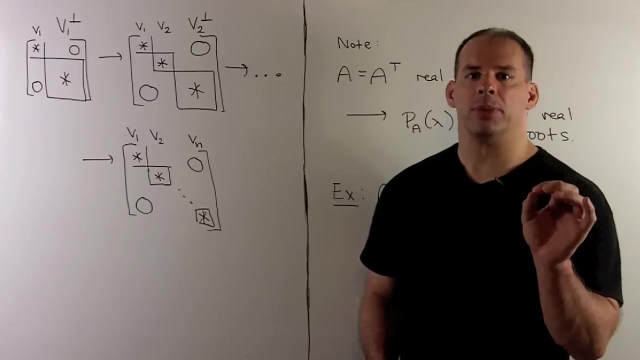 keep choosing successive vectors from the orthogonal complement. Now that means I have an orthogonal basis of unit vectors, so we have an orthonormal basis of eigenvectors for a, and that's our result. We can picture our recursive process by considering the matrix A at each step. So in the first step we have a non-zero eigenvector. 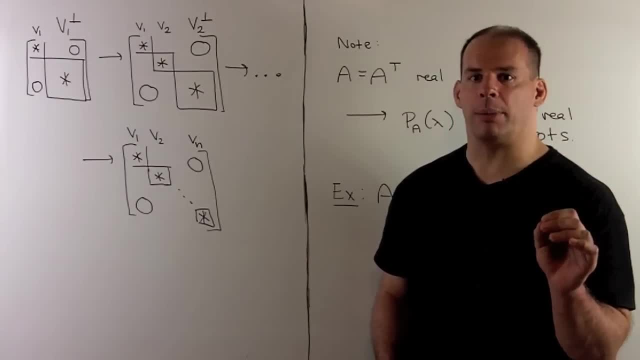 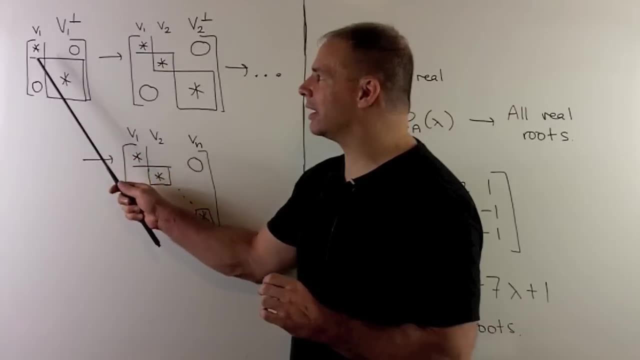 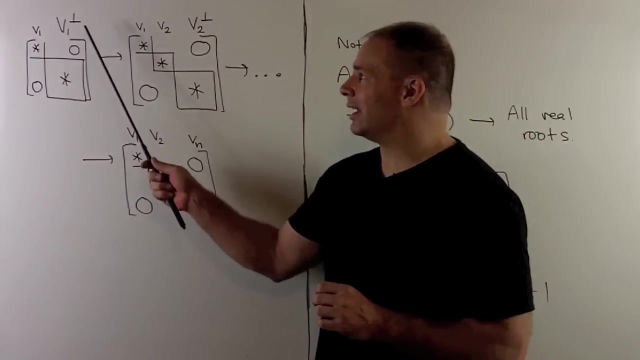 V. Take its span form, its orthogonal complement. We choose our basis correctly, We'll have a block diagonal matrix with a one by one block in the upper left hand corner representing our eigenvector. Then I could choose non-zero eigenvector in the orthogonal complement and repeat. 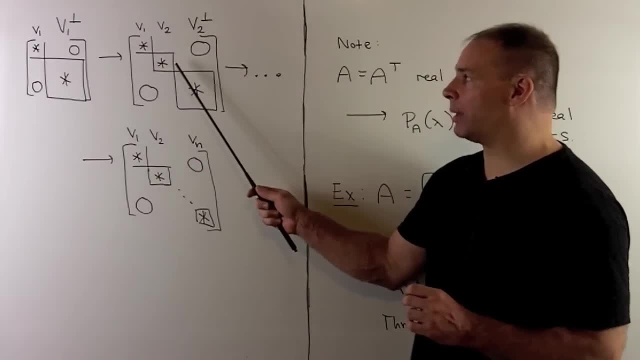 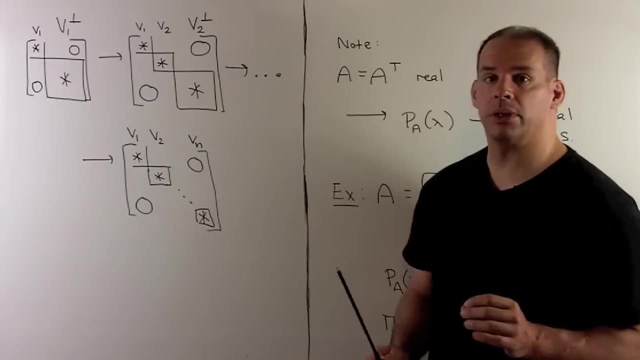 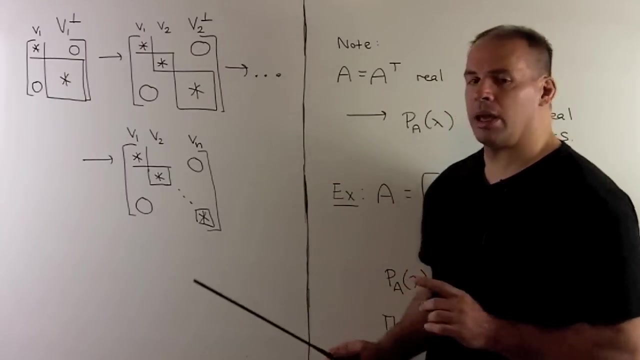 So we'll have block diagonal with two one by one blocks, and then we'll have an n minus two by n minus two block, representing the new orthogonal complement. We repeat this process until we squeeze this large block down to a one by one block and what we're left with is a diagonal matrix that represents A.